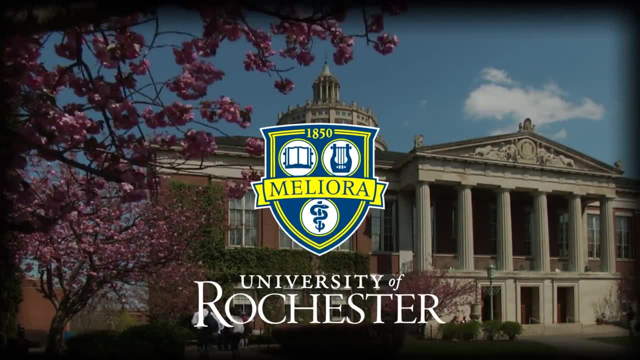 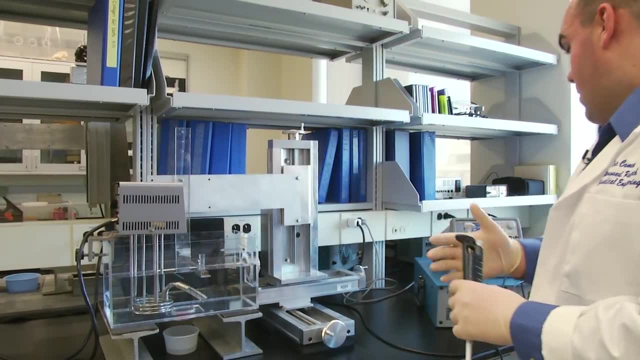 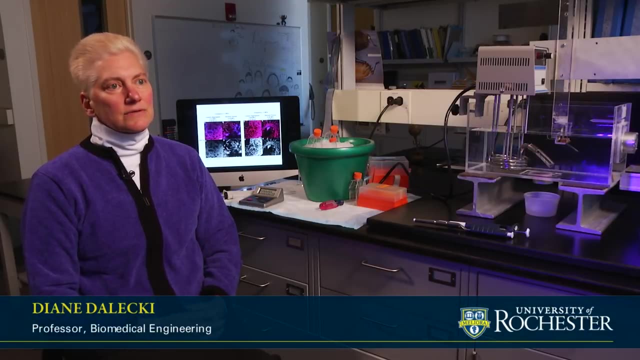 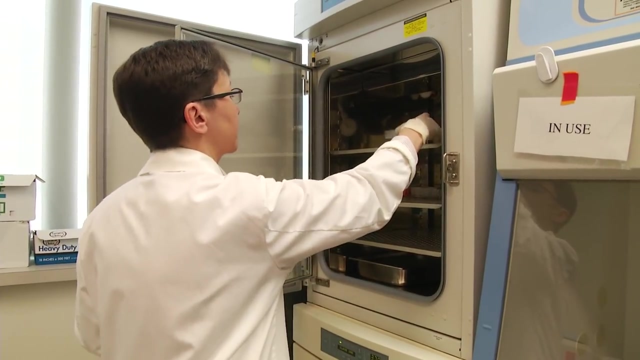 In our laboratories we're developing new ultrasound-based technologies to advance this field of tissue engineering. The long-term goal of tissue engineering is to fabricate living, functional artificial tissues and organs. I got involved because Diane contacted me, probably a good ten years ago, saying she was interested in wound healing. 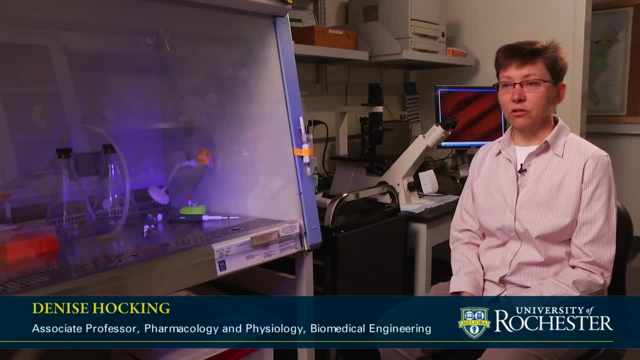 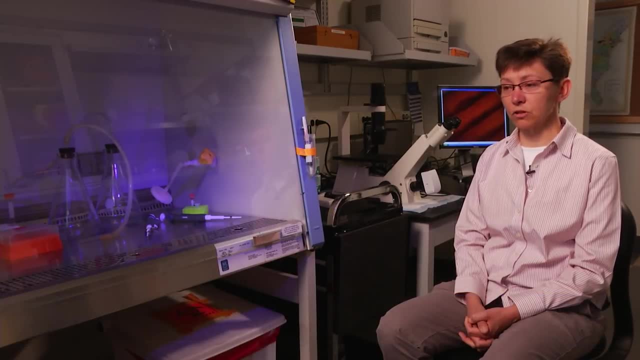 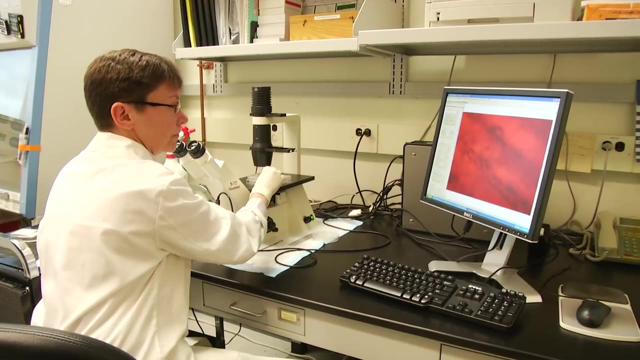 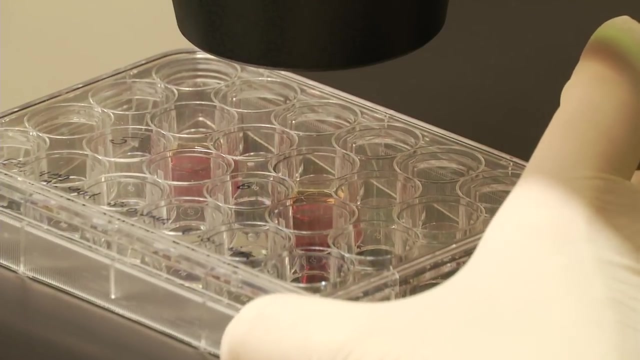 So I was looking at the biological mechanisms involved in wound healing and Diane had seen some lectures concerning how ultrasound might enhance wound healing And that suddenly a light ball went off in my head and I said, if it's a simple force and we can, it's kind of like you could whisper on a cell and affect the way the cell functions or the way the proteins are laid down. 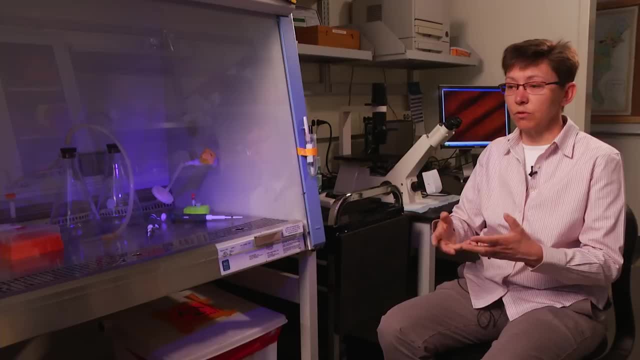 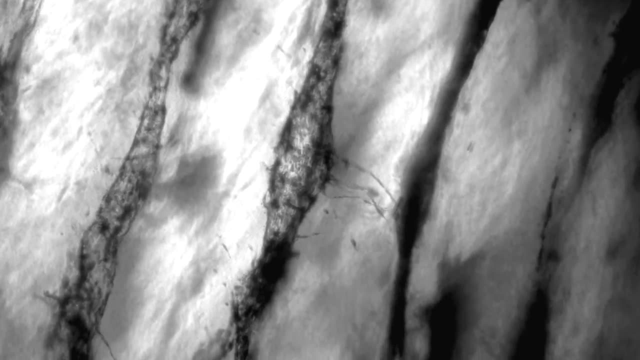 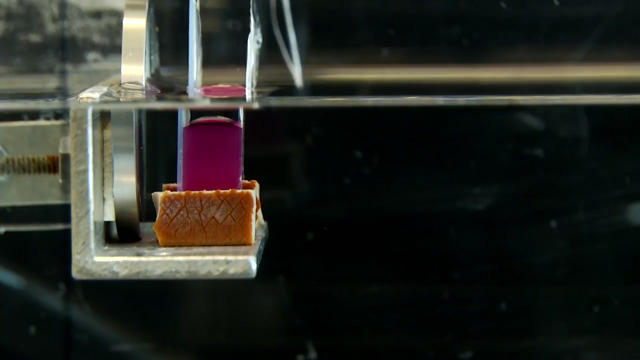 then maybe we have the opportunity to be able to control cells, control tissue organization, simply by exposing them to different ultrasound parameters. Here I have an ultrasound set up Right now. I have particles suspended in water and when I activate the ultrasound it will non-invasively pattern these cells into planar bands. 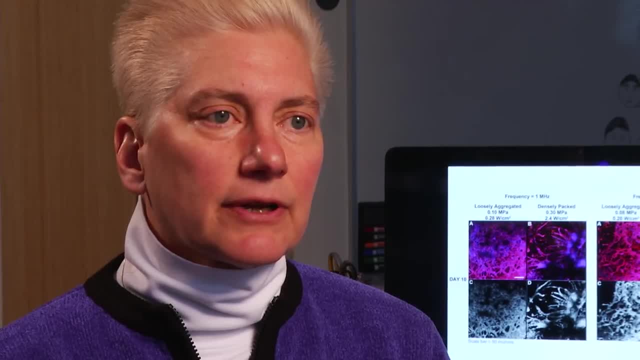 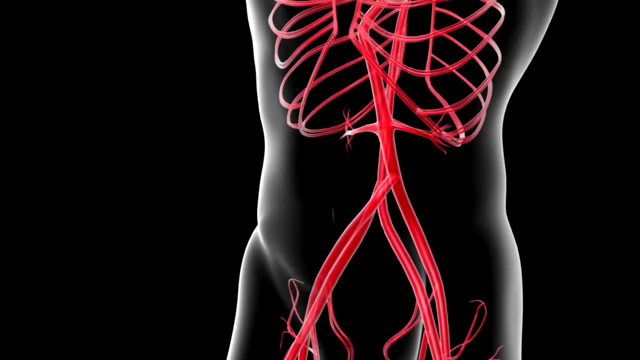 One particular challenge that I have is that I don't know how to do it. One type of tissue that we're focused on right now is creating micro-vessels, creating a vascular network in the tissue. As we know, all tissues need a vascular network in order to survive right. 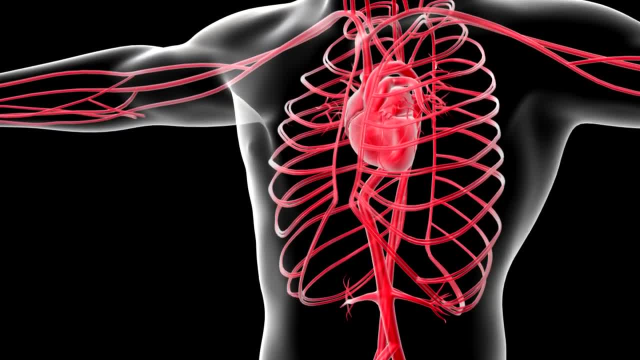 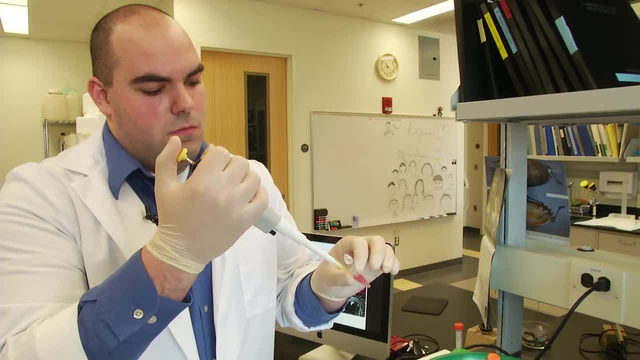 The vascular network is what brings the nutrients to the cells and takes away the waste products. You might think of the ability to create a vascular network in an artificial tissue as one of the largest challenges in tissue engineering, And solving that is perhaps sort of maybe the holy grail of tissue engineering. 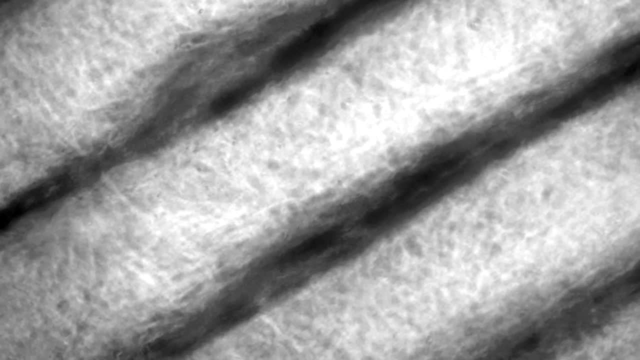 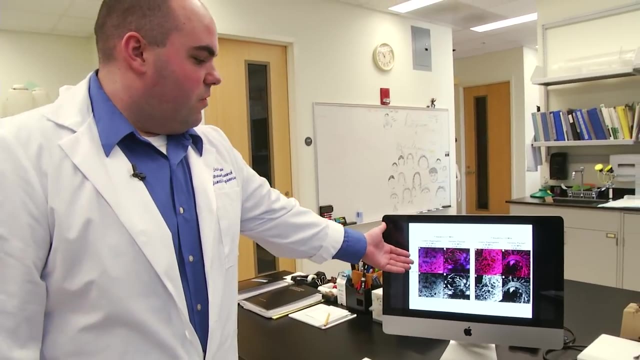 When we use endothelial cells, we don't know how to do it. When we use endothelial cells, which are the cells that form blood vessels in the body, we have shown that they form vessels, as shown here, So we can make both capillary-like networks as well as thicker branching vessels.